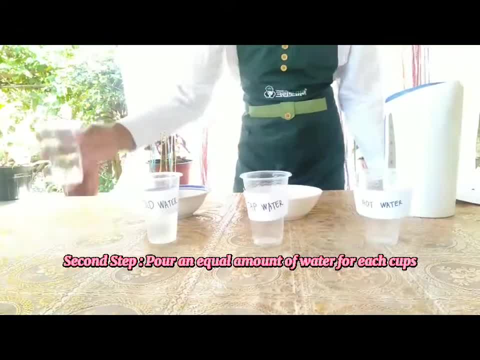 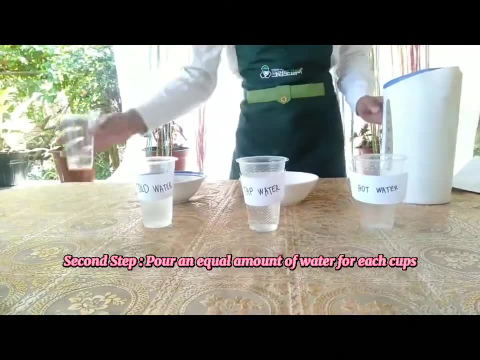 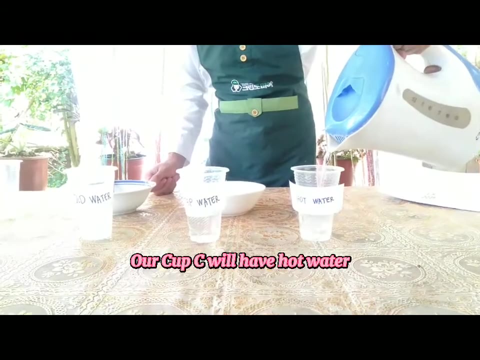 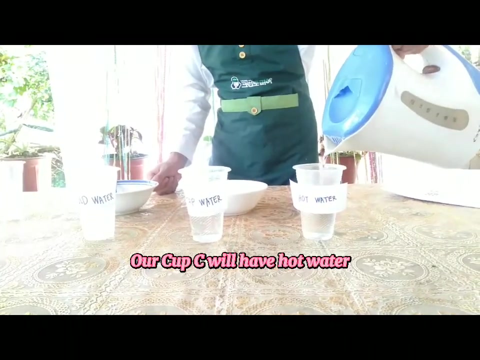 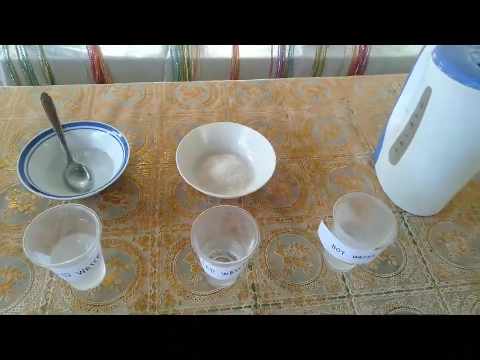 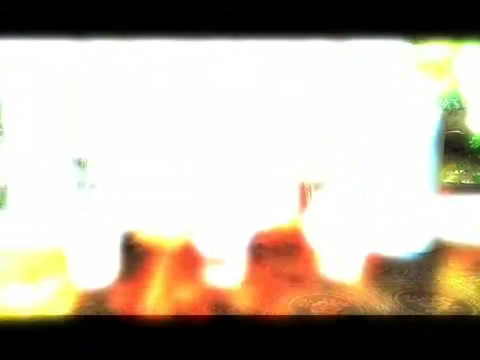 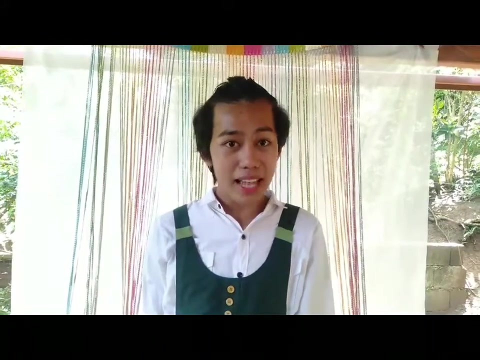 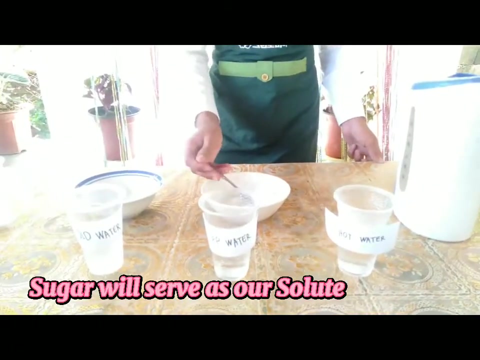 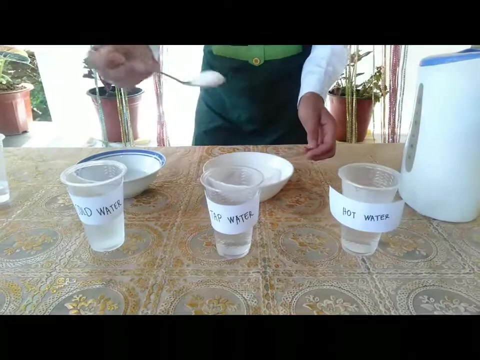 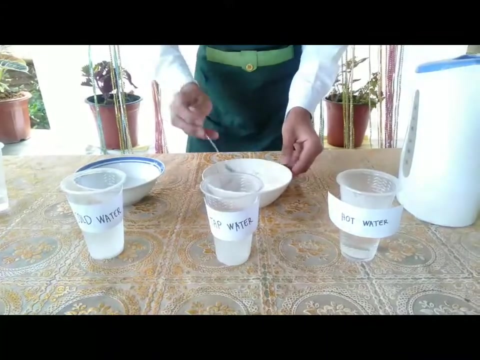 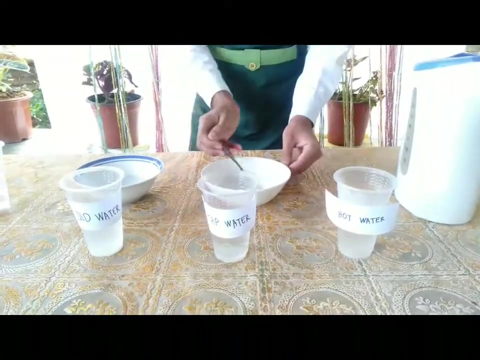 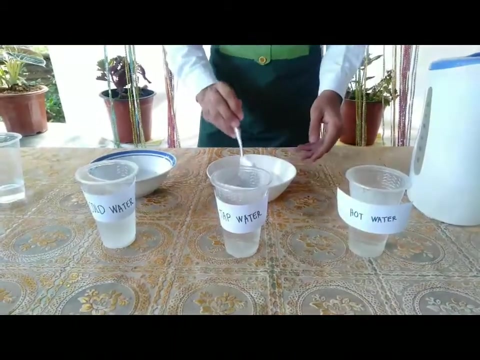 So, So, So, Hey, So, Now, Now, And after pouring an equal amount of water to each cup, now we're going to pour the apply solute, which is sugar, on each cup. Okay, We're going to put it in one cup of water. 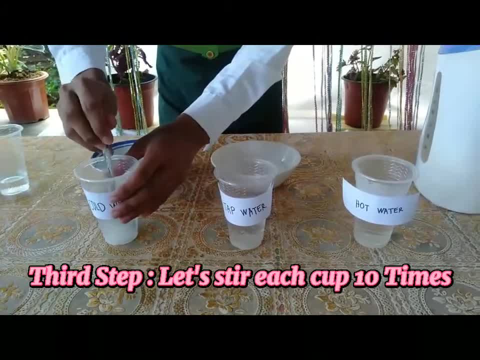 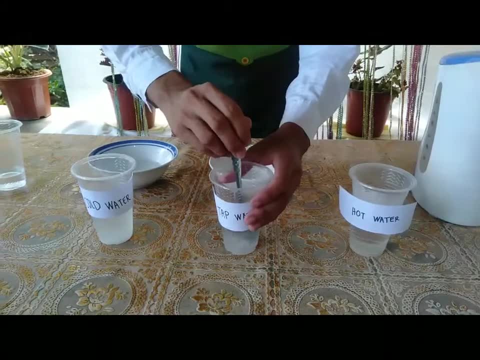 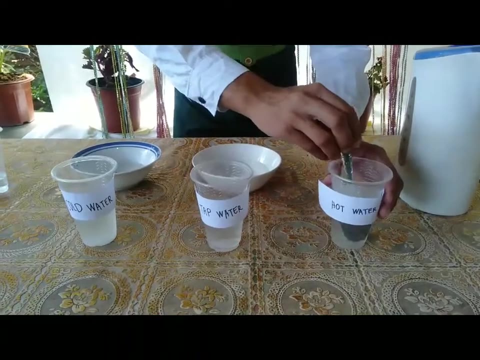 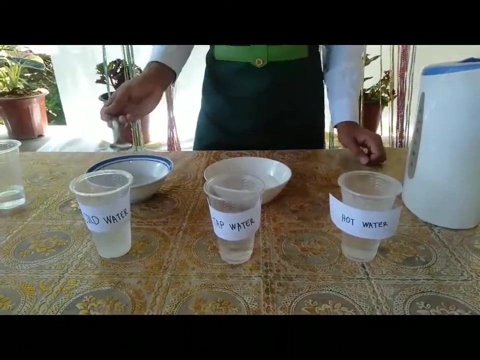 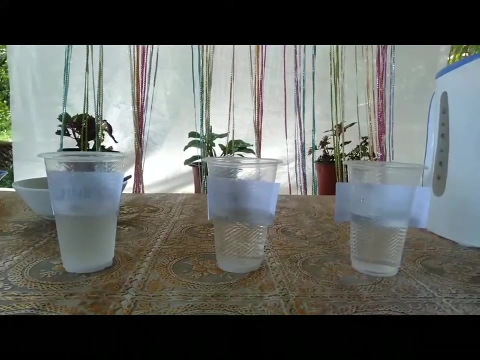 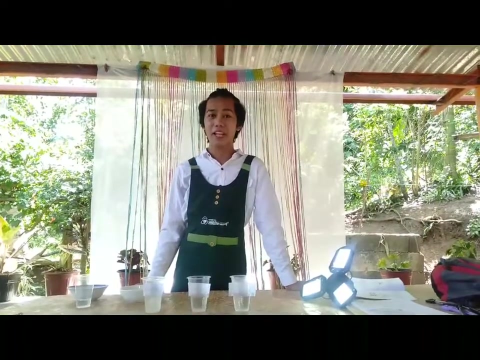 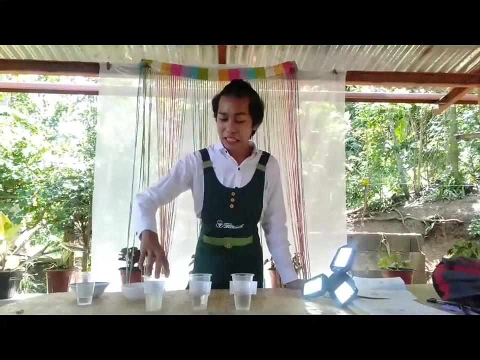 Okay, And you want to let Bring in all the water to the cup? Okay, Good, Let it. Hey. After observing our experiment, we're going now to know the result. Okay, so this is the cold water. The cold water doesn't dissolve much. 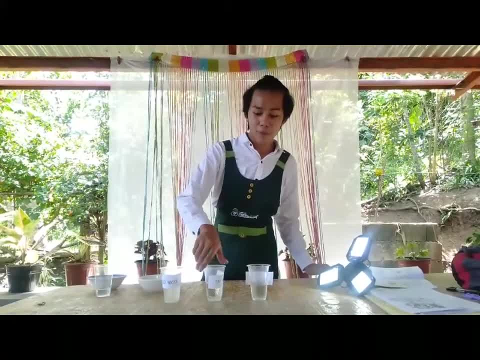 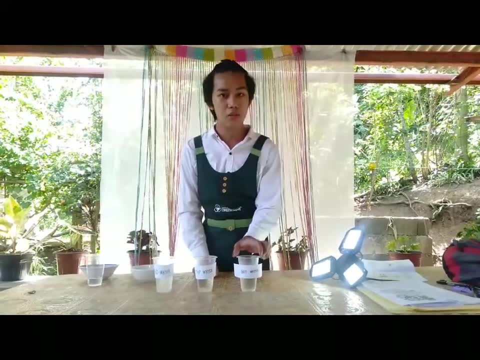 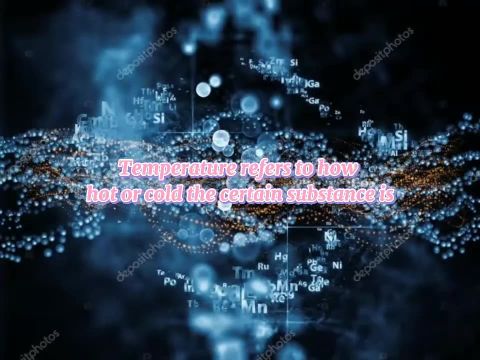 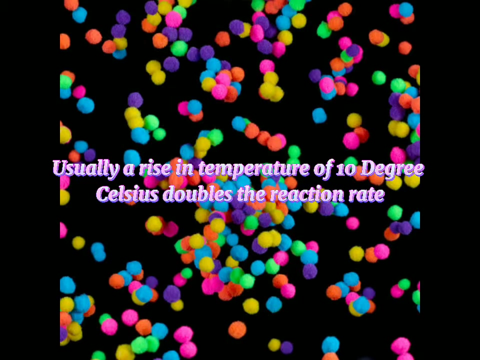 Our solute, Then this is the tap water And this is our hot water, which dissolves totally the solute or the sugar that we put in. this Temperature refers to how hot or cold the certain substance is. Usually, a rise in temperature of 10 degrees Celsius doubles the reaction rate.